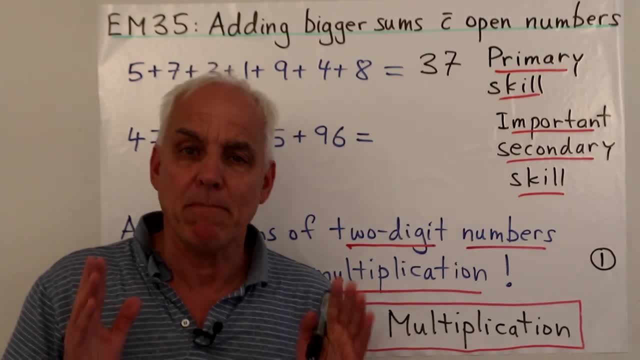 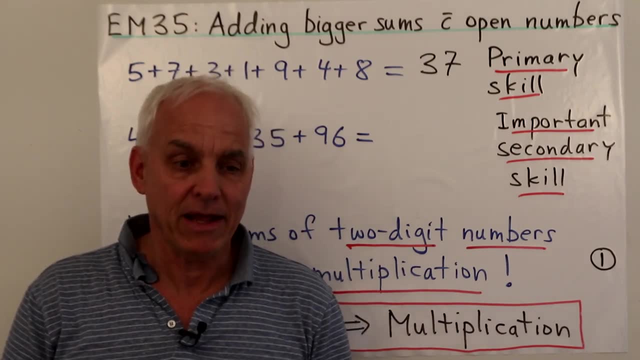 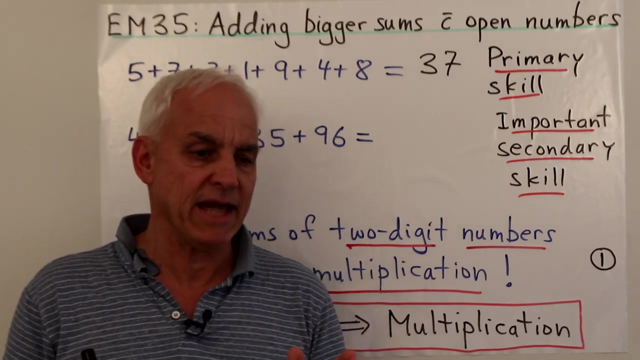 and quantitative subjects more generally will become much simpler for them. And it's probably good for me to reiterate what I've often said, but it's worth repeating that in this approach, calculators play absolutely no role. So at no point should we say, oh, but 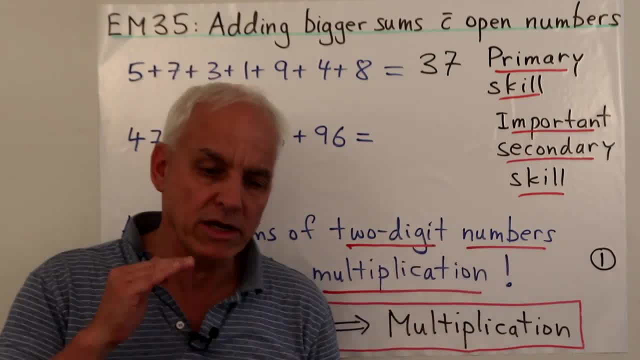 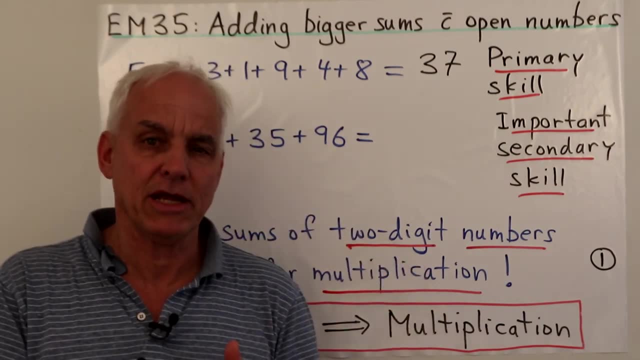 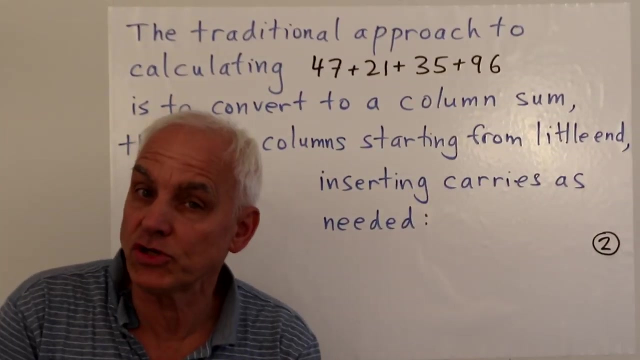 wait a minute, calculators can do this job. No, We want to make sure our students are able to successfully, confidently, accurately perform this fundamental kind of arithmetic, Absolutely crucial Now. the traditional approach to teaching students to sum up something like this is to first of all convert it to a column. 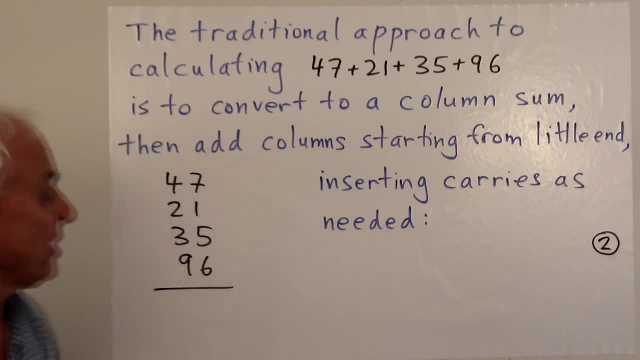 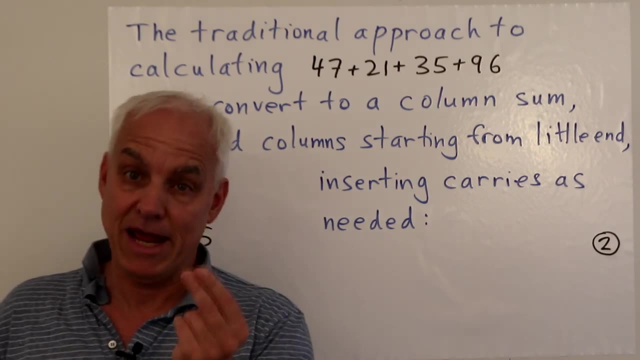 sum. So we arrange the numbers of the column one on top of the others, with ones aligned and the tens aligned and so on, And then we start adding the columns from the little end, That is from the ones column first, And then we move from right to left. First the ones, 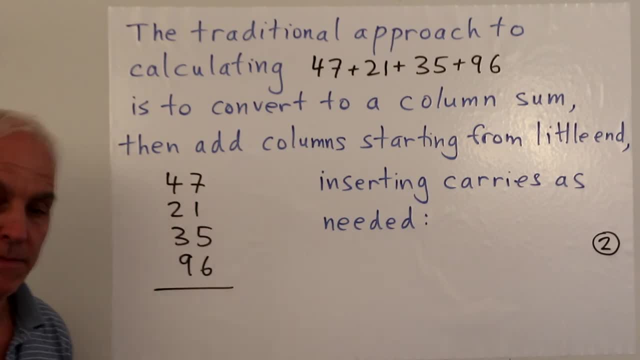 column, then the tens column, then the hundreds column, and so on, And as we go we insert these columns from the問 column. We just sort this out, so this week will be easy. So for example, here we would add the ones: Seven plus one is eight, plus five is 13,, plus six is 19.. 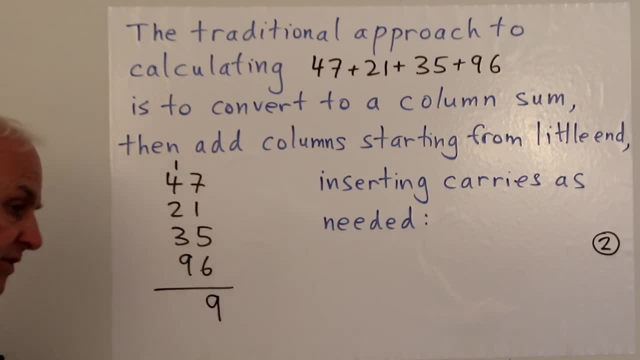 So we write the nineteen with a nine here, and then we add a little one kind of kind of a superscript on top of that next column. That's then added to the total here. So we get: one plus four is five plus two is seven plus three is ten plus nine is 19.. And the nine comes here. 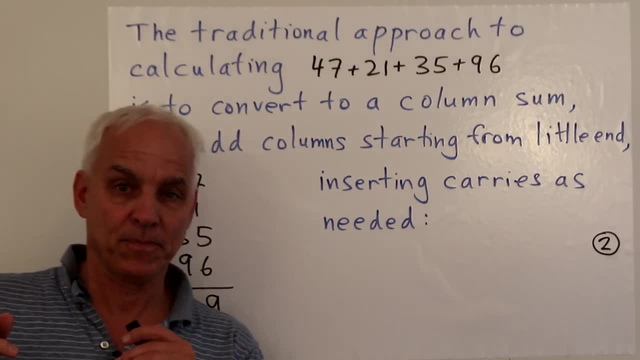 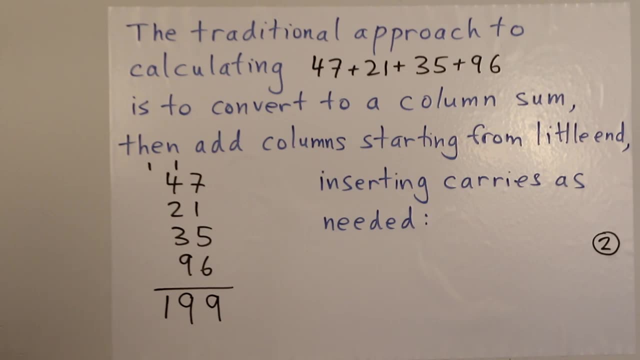 and the one officially goes into the next column, And then the one even вообще 이렇게 column. now there happen not to be any other entries in that next column, so the one just comes down and we get 199. that is the standard approach, from right to. 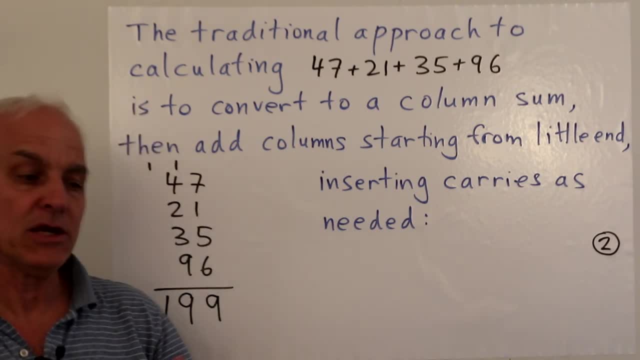 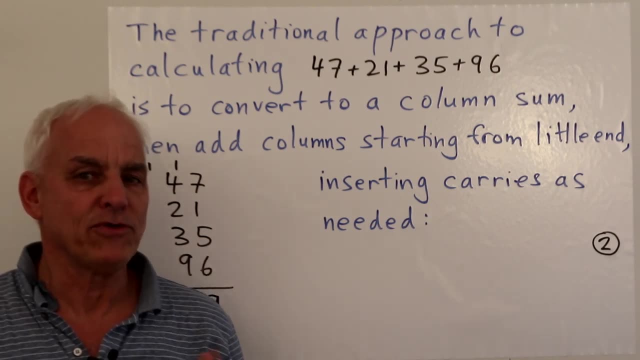 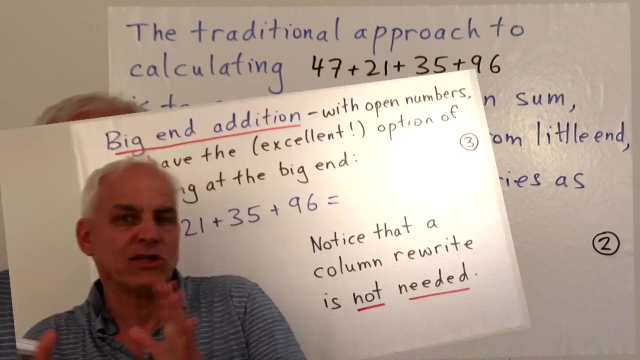 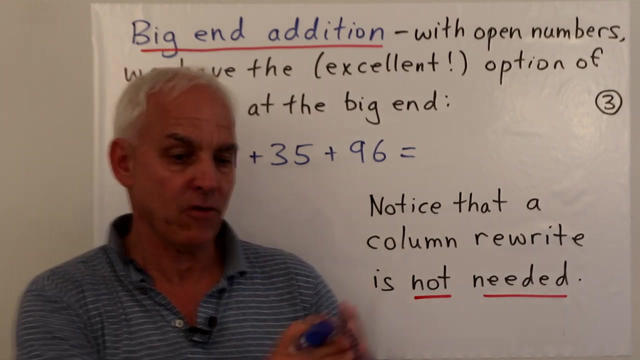 left. in other words, starting from the little end and interspersing summings with carryings. we want to move to a slightly different point of view, I think a preferable point of view. now, okay, we're going to slowly be making this shift from a little and orientation to big and orientation instead of. 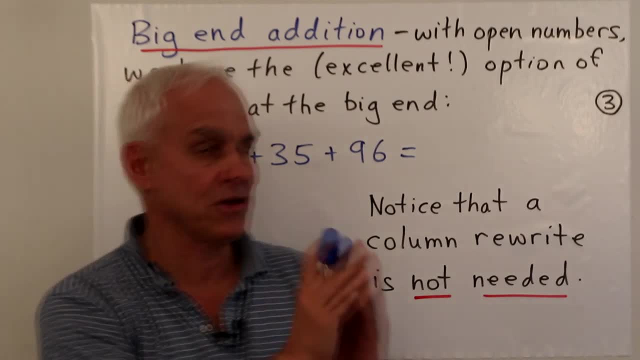 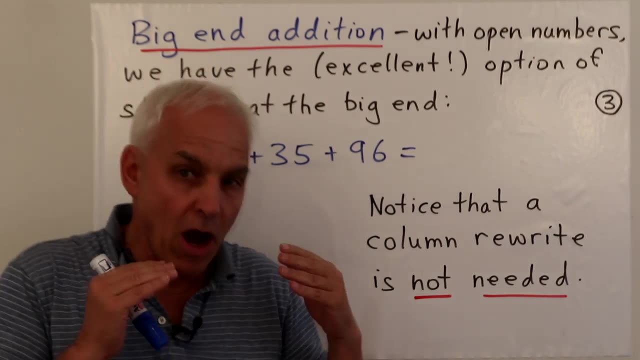 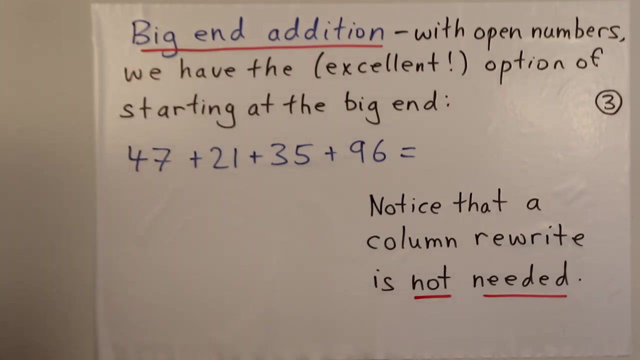 proceeding from right to left. we're going to proceed from left to right, so with open numbers, we are in a position to do this with ordinary Hindu Arabic numbers. there are obstacles to doing this. that's one of the advantages of open numbers: they allow us to consider this big end approach, tradition. so let's 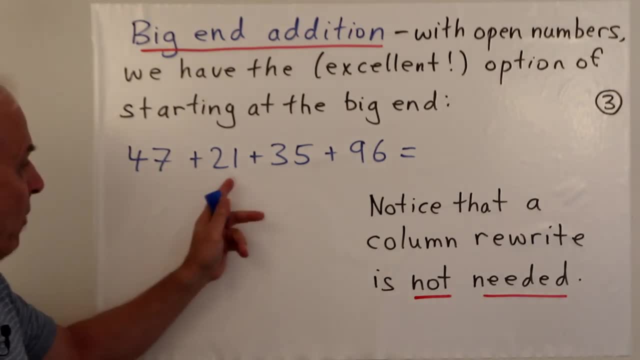 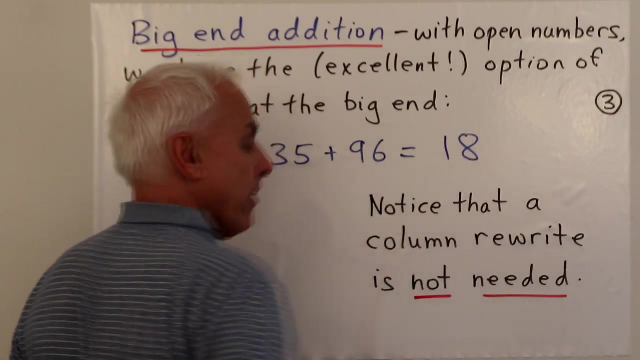 illustrate that. here's the same sum: 47 plus 21 plus 35 plus 96. we start from the big end, which is the left most digits, the tens in this case. we add up the 10's: 4 plus 2 is 6, plus 3 is 9, plus 9 is 18 and we write the 18 there. it's natural, it's the. 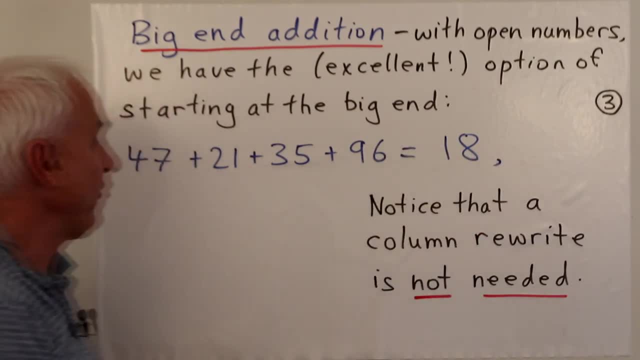 next thing that we write. then we write a comma and we proceed to summing the ones entries: 7 plus 1 is 8, plus 5 is 13, plus 6 is 19. so we've obtained an open number by doing this big end addition. now, if we want to convert that to a regular number, we are 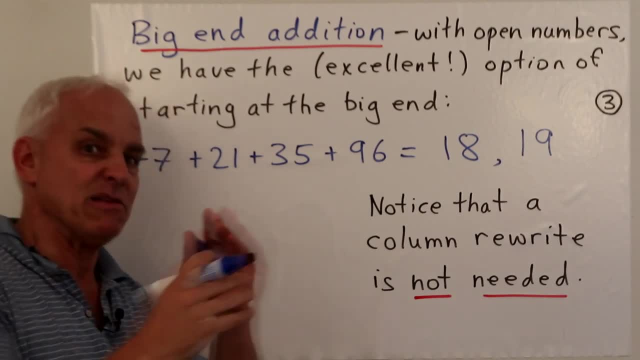 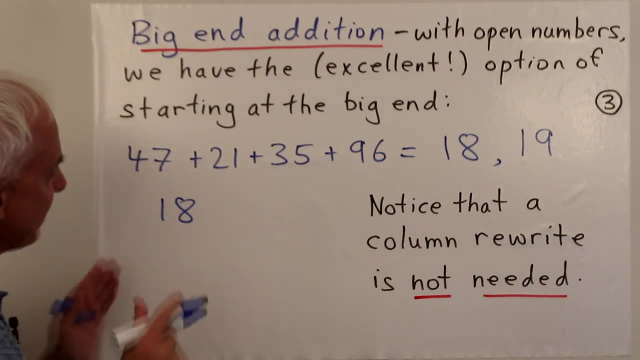 going to do a cascading, but we're going to maintain this big end point of view, starting with the 18, and then the 19 is going to be juxtaposed to the right, because this 1, 8 is occupying the, the tens column and the hundreds column, the 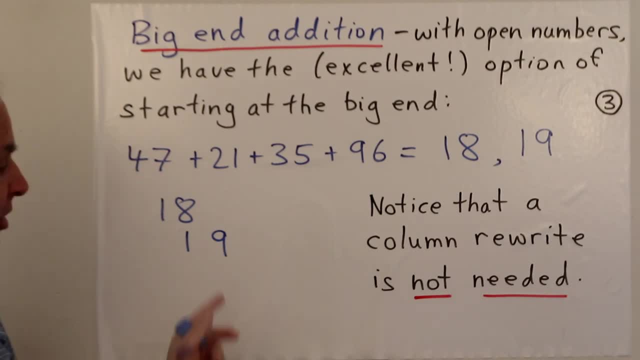 19 that we're going to write will be put over here, occupying the ones and the tens column, so it's a little bit different from what we had before. now the cascading goes like this, and then we can add 1, 8 plus 1 is 9- 9, and we get the same answer as we did. 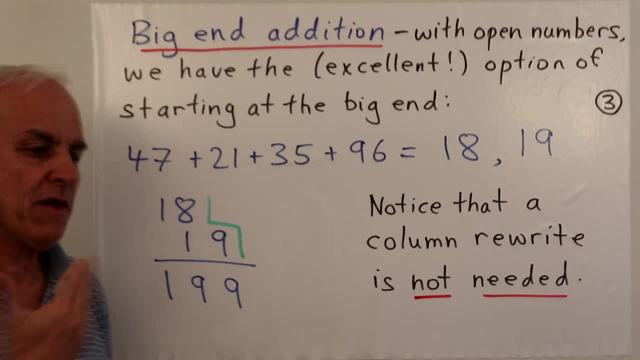 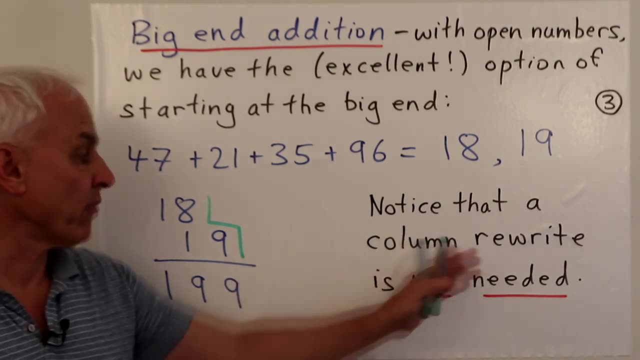 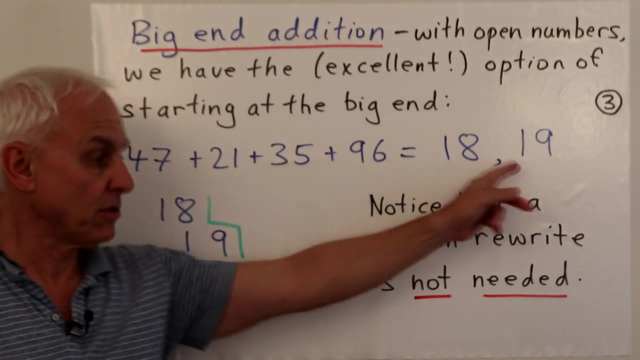 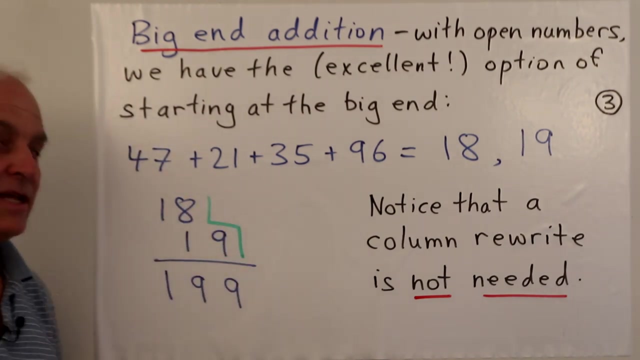 before. but we're starting from the big end and notice that with this approach another advantage is that a column rewrite is not needed. we can proceed very pleasantly with this row form to go directly from that to the open number. then we have to employ a secondary process to convert that, the cascading. 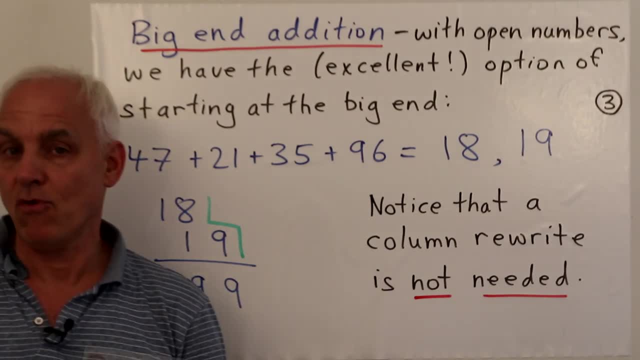 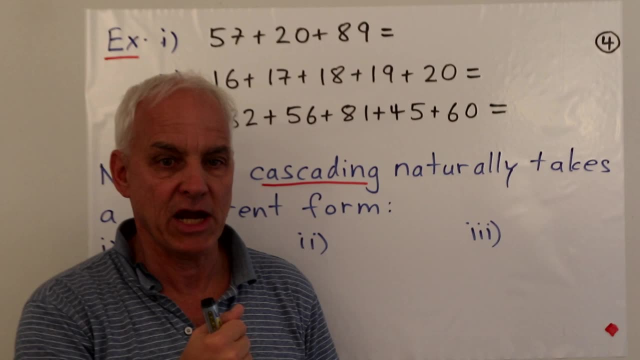 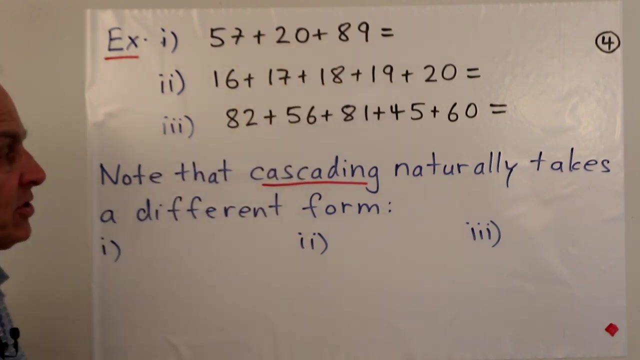 phenomenon to our more standard Hindu Arabic form. alright, let's get some more practice. summing up these slightly bigger numbers with this big and orientation, proceeding from left to right: 57 plus 20 plus 89. we start with the big end: 5 plus 2 is 7 plus 8 is 50. 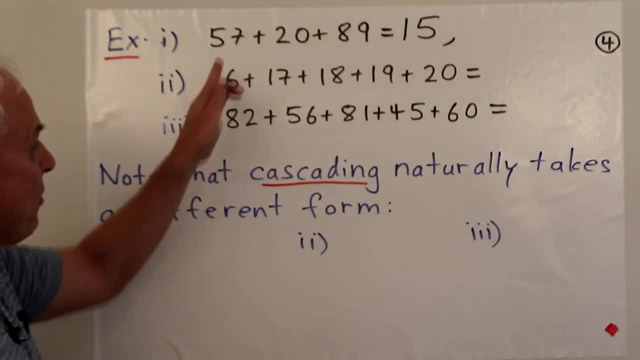 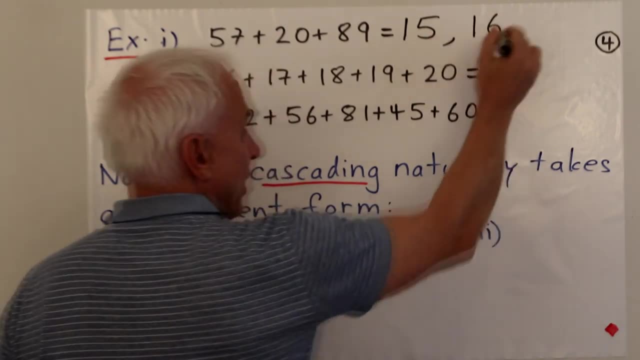 We write the 15 and put a comma. Now we move to the ones: the 7,, the 0, and the 9.. 7 plus 0 is 7, plus 9 is 16.. So there's the result as an open number. 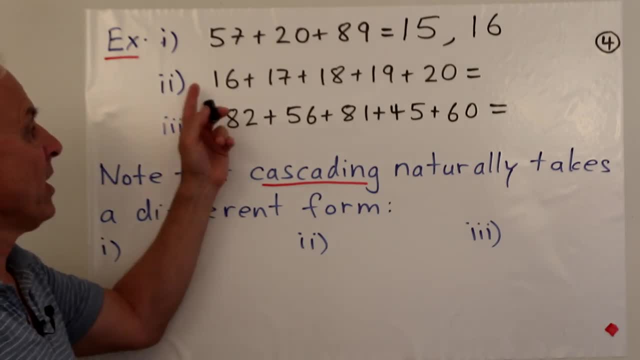 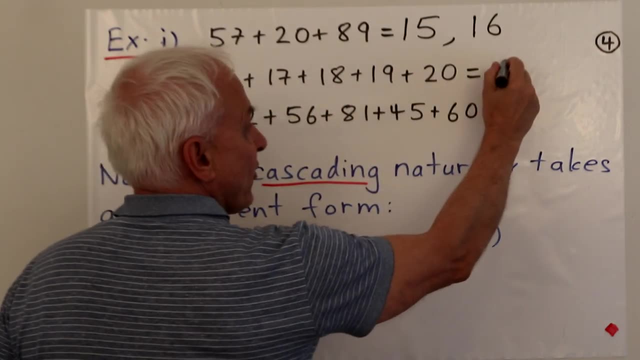 Let's leave it like that for now. How about here? 16 plus 17 plus 18 plus 19 plus 20.. Starting from the big end, 1 plus 1 is 2, plus 1 is 3, plus 1 is 4, plus 2 is 6.. 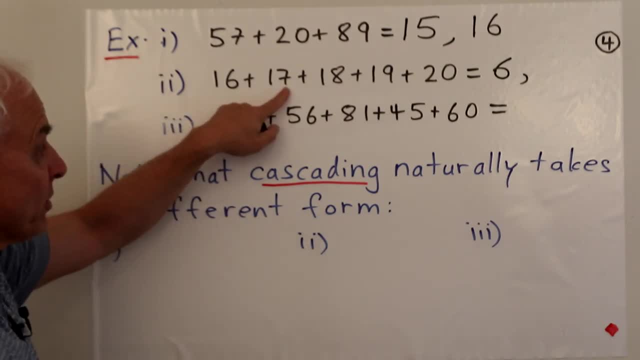 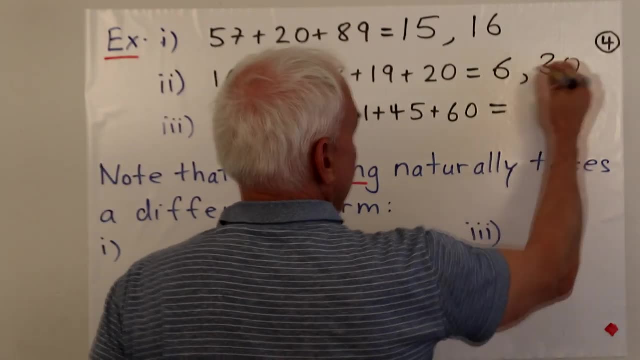 Then we put a comma, Then 6 plus 7 is 13,, plus 8 is 21,, plus 9 is 30,, plus 0 is still 30. There's the result as an open number: 6, comma 30.. 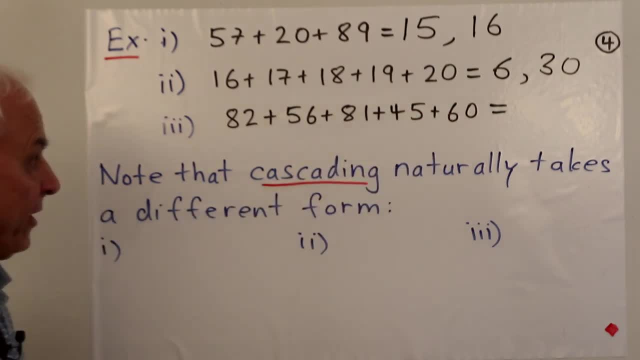 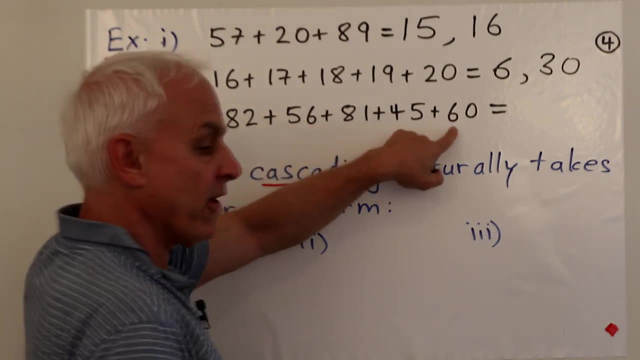 Here we have 82 plus 56 plus 81 plus 45 plus 60.. 8 plus 5 is 13,, plus 8 is 21,. plus 4 is 25,, plus 6 is 31. Comma. 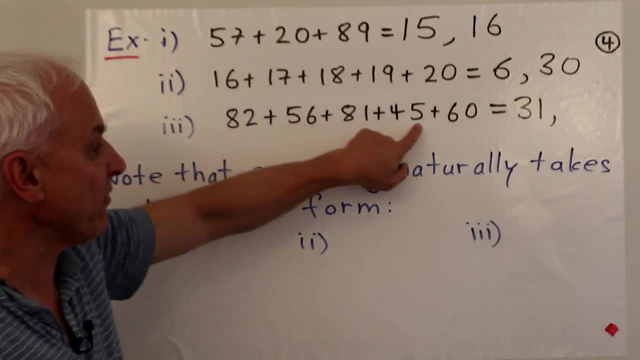 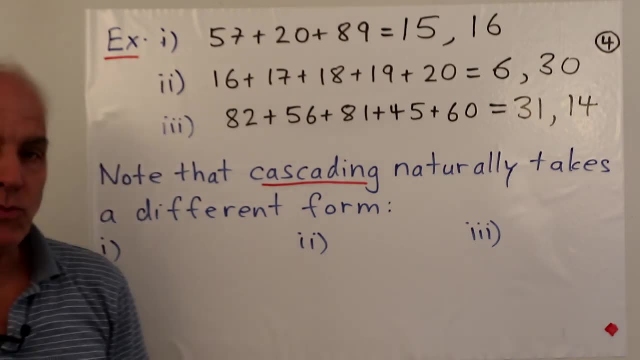 Then the ones: 2 plus 6 is 13.. 6 is 8, plus 1 is 9, plus 5 is 14, plus 0 is still 14.. So, of course, we're leaning very heavily on our fundamental ability. 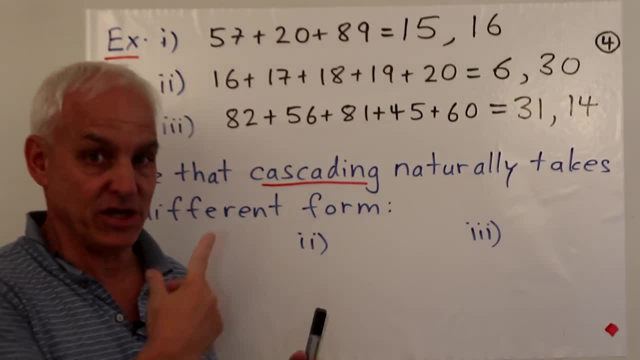 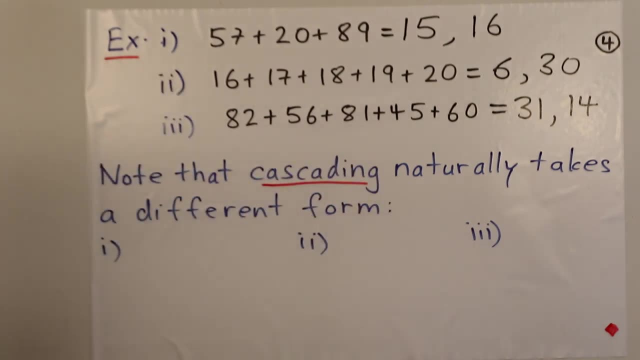 to be able to sum a bunch of single digit numbers, Perhaps quite a lot of them, Involving wrapping around 10 and 20 and 30 and so on. Okay, but we're not really finished here, because we only have open numbers at this point. 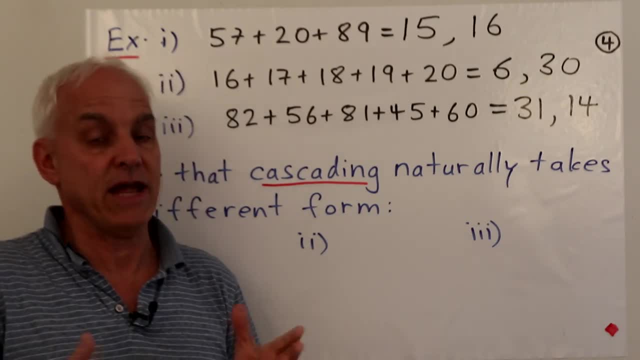 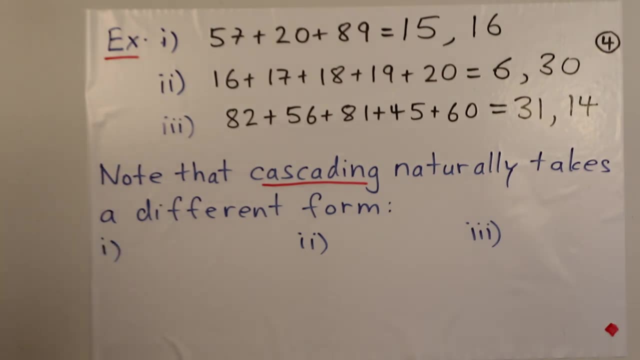 We'd like to further convert, Convert those into standard Hindu-Arabic numbers. So let's do that again. But I want to then show you, emphasize, that the cascading that's happening is a little bit different from previously, because we're still maintaining our big end point of view. 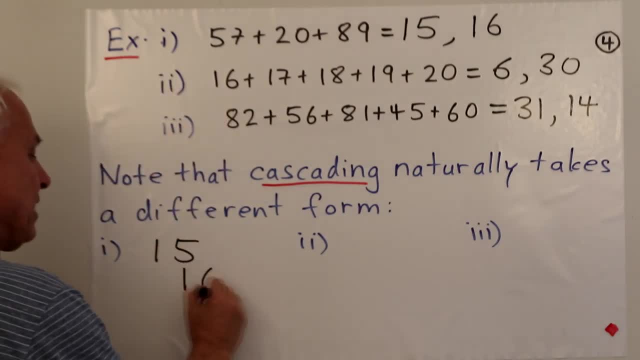 So 15, 16.. We write the 15 and then we write the 16 below it, Summing 1,, 6, 6.. How about over here? We write a 6. And then we write 30.. 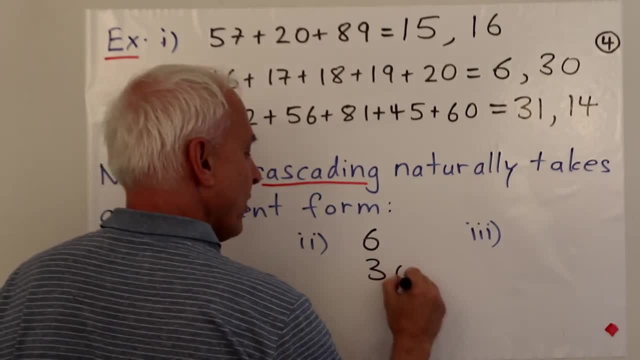 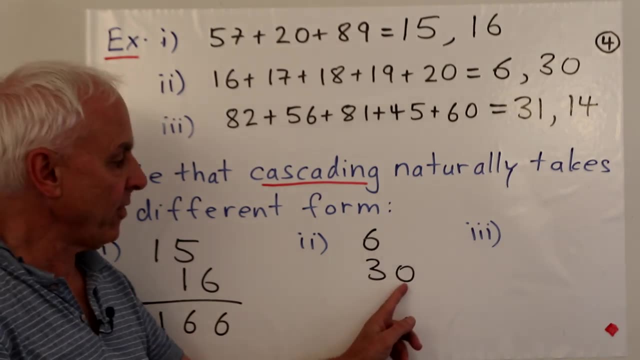 So where does the 30 go? The 30 goes like this: The 6 is really the total number of 10s, The 30 is the number of 1s In the 1s spot, that's, in the 10s spot. 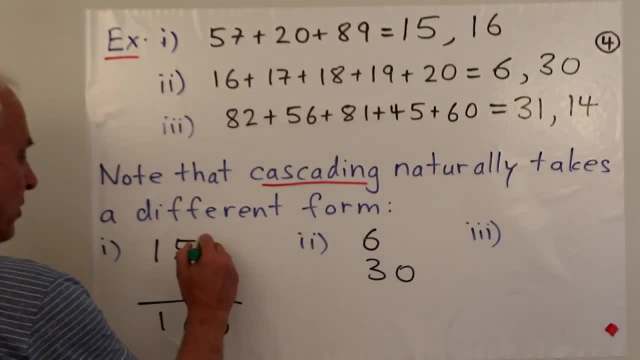 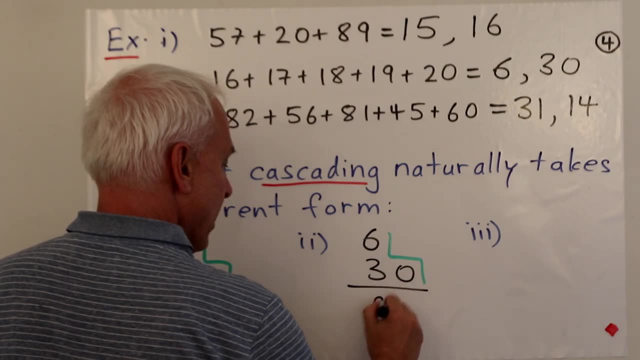 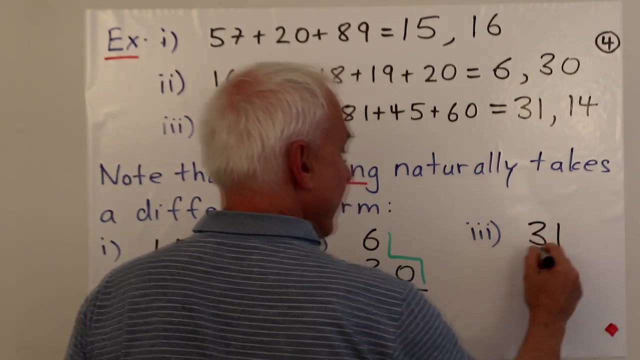 If we want to actually illustrate cascading, we would do it like this, Like this: Okay, now, when we add these, we get 9 and 0. And finally, 31 and 14.. 31, that's the number of 10s and 14 is the number of 1s. 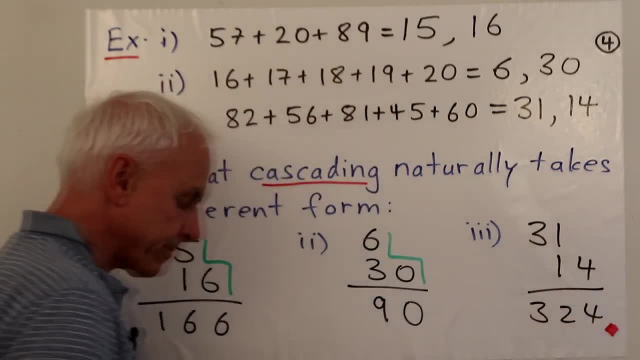 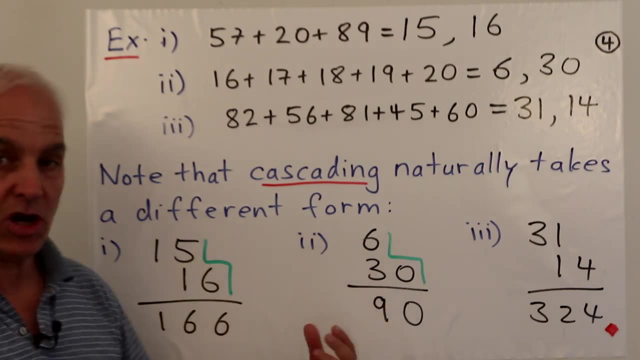 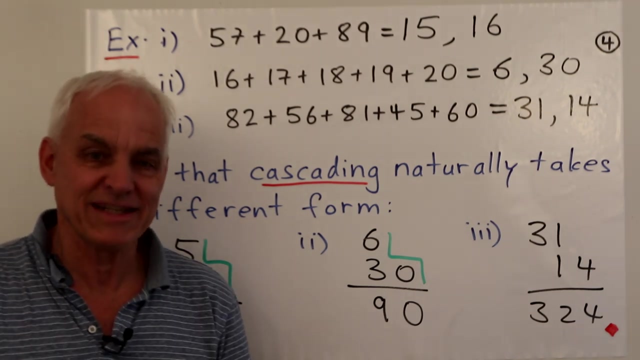 We get 3,, 2,, 4.. Now these are all in some sense kind of simple because we have not had any sums which are bigger than 9.. If we got some of those, then we may have to do a further simplification to get a Hindu-Arabic number. 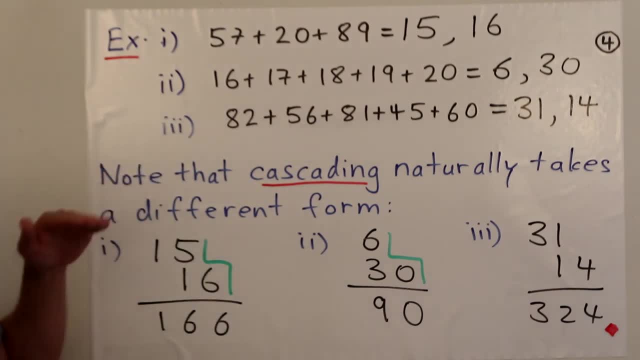 Hindu-Arabic number. Okay, so we see quite a distinction here between the summing process just involving all of the lanes separately, starting from the big end. That just involves our basic technology of adding digits completely separate, with essentially no carries We end up. 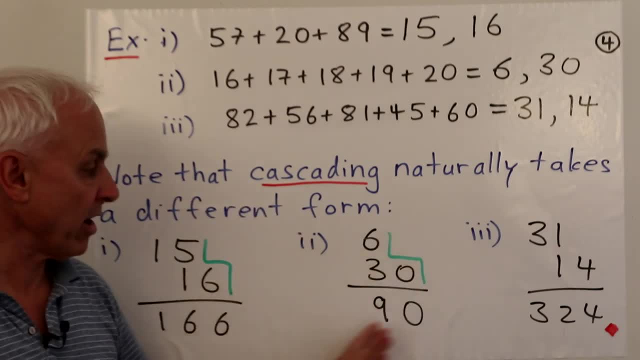 getting open numbers, and then we convert the open numbers into Hindu-Arabic numbers, with a cascading approach, but now slightly differently, because we're mating the big end approach and writing the- in this case the tens- first and then the ones. 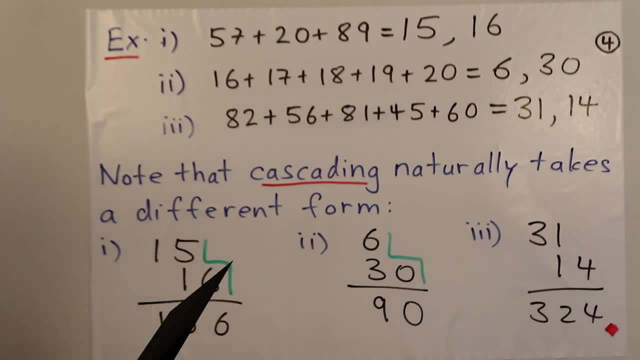 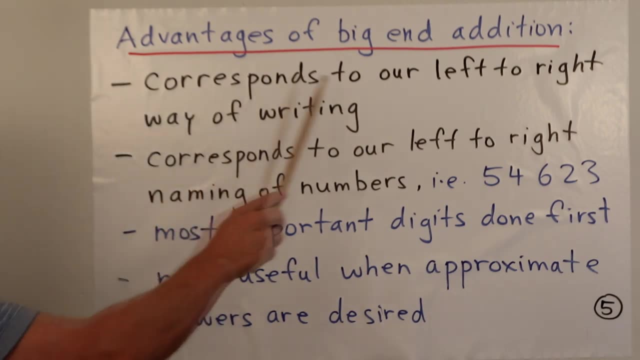 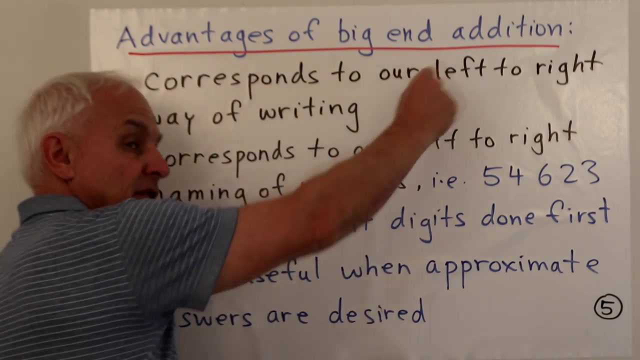 below that and to the right. So what are the advantages in working with this big end approach to addition? Well, first of all, it corresponds more smoothly to our left-to-right way of writing. When we write, we start from the left and we proceed to the right. 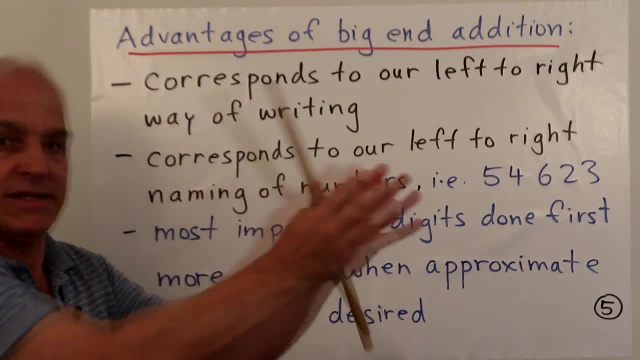 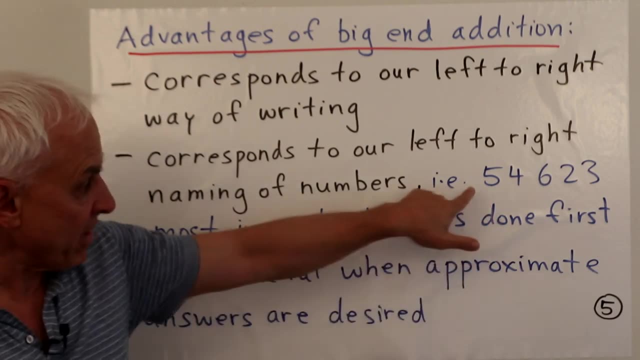 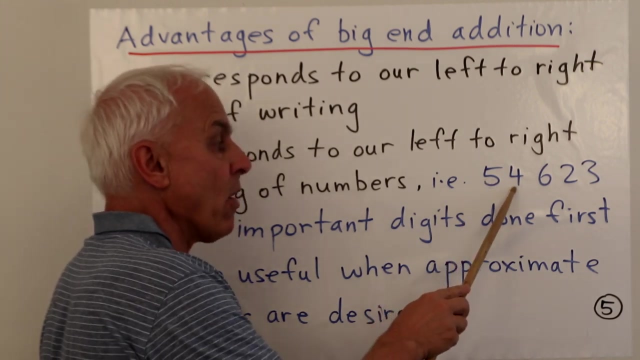 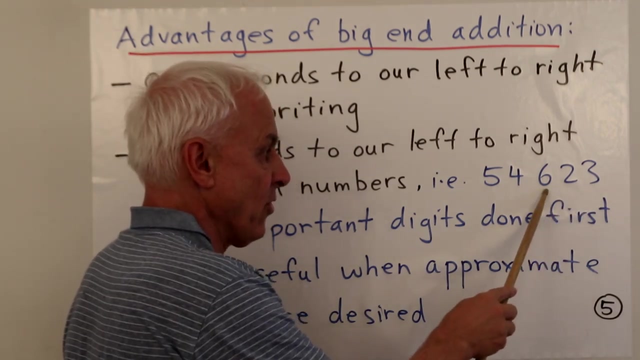 So this naturally aligns with that basic orientation. It also corresponds to our left-to-right naming of numbers. If we have a number like this, how do we read that? How do we think about this number? We say this is 54,623.. We don't say it's 3 and 20 and 600 and 4,000, and 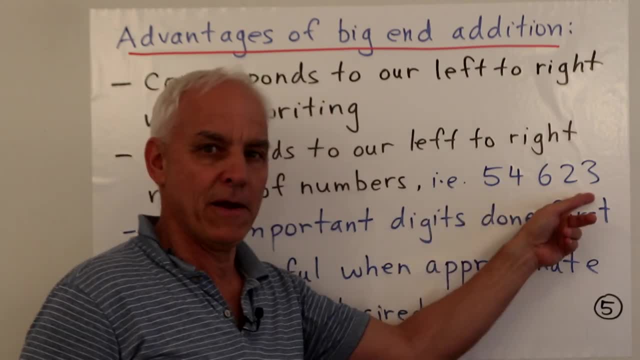 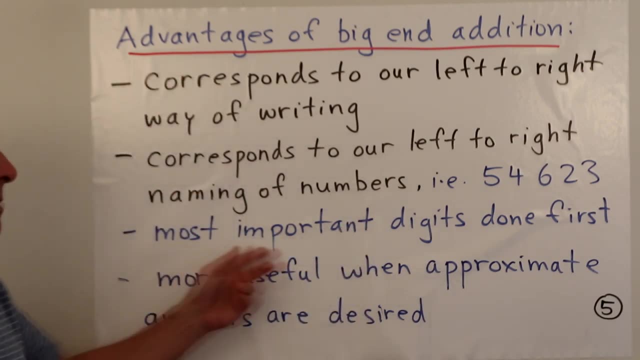 50,000,. right, We proceed this way. That's the same direction that we're going here with this big end approach. We're starting from the biggest digits. Okay, the most important digits, namely the ones to the left, are done. 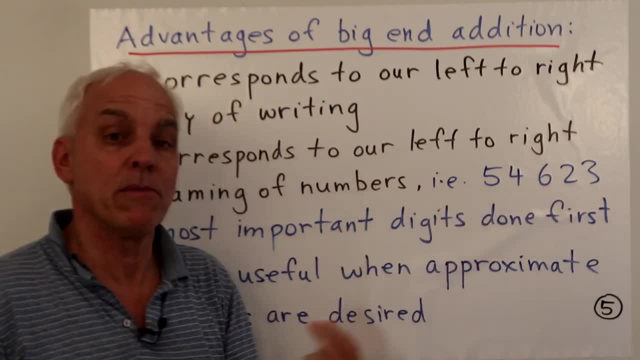 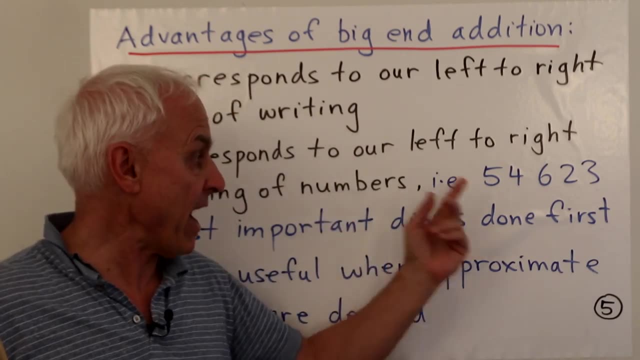 first With a number like this, the most important digit here is the 5, because that's representing the biggest unit- the 10,000s, and then after that the 4,, and then after that the 6,, and then 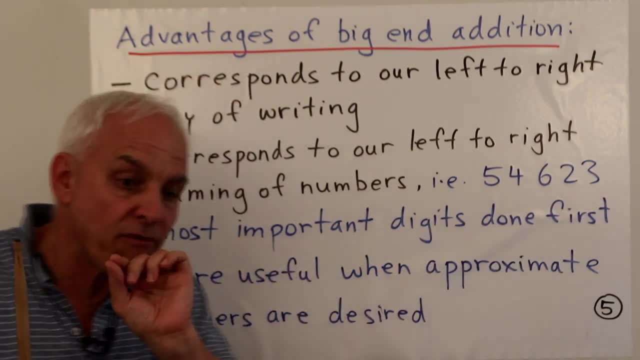 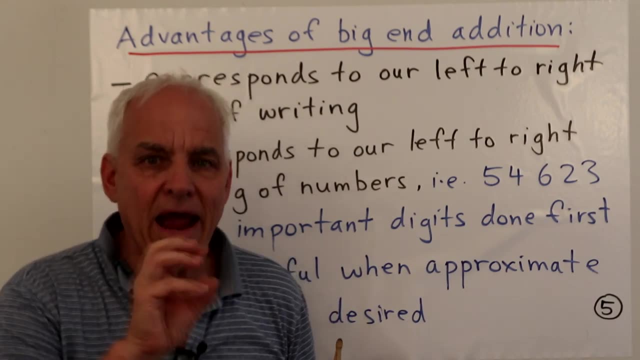 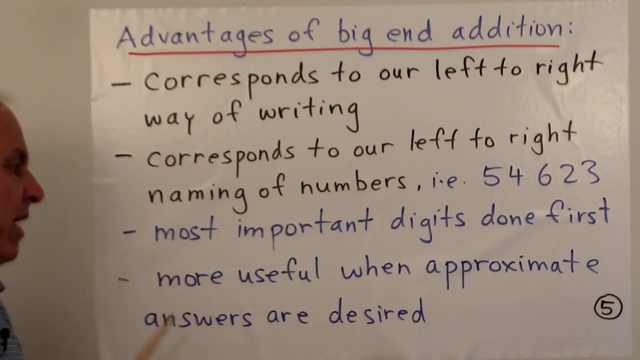 after that the 2, and then after that the 3.. As we move from left to right, the digits are becoming less important. They correspond to finer and finer detail. okay, Another way of saying that is that this is more useful when approximate answers are desired. 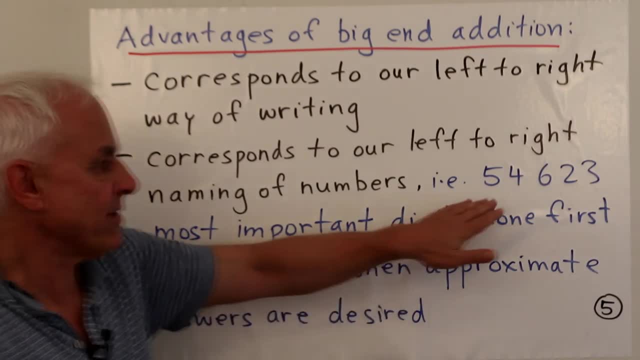 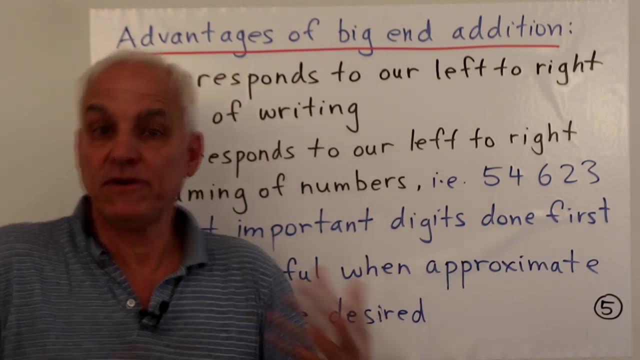 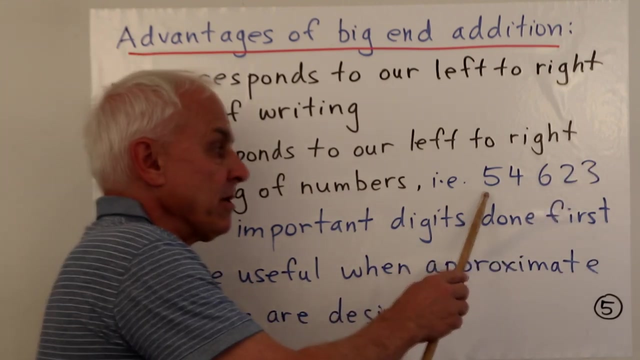 Let's say we were not that interested in what such a number is exactly, but just approximately. So approximately, we could say: well, it's roughly 54,000.. Or maybe we could say that's approximately 50,000. Or maybe it's approximately 54,600.. In all of those cases, what we're doing is we're. 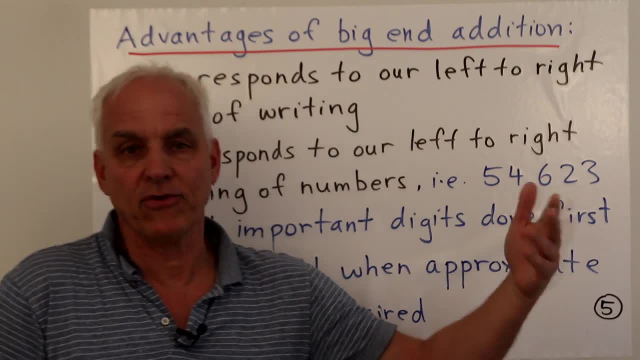 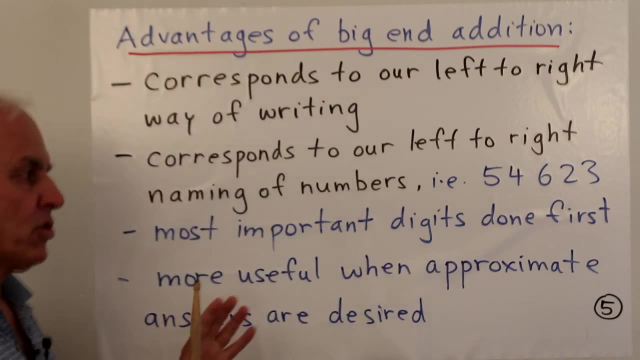 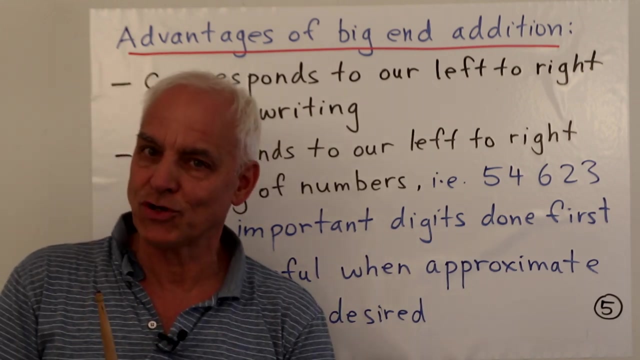 dropping some of the rightmost digits and considering them sort of negligible or relatively unimportant. okay, So our big end approach is in line with that which is really in line with sort of a scientific approach to measurement. I want to say a little bit more about the number of digits. 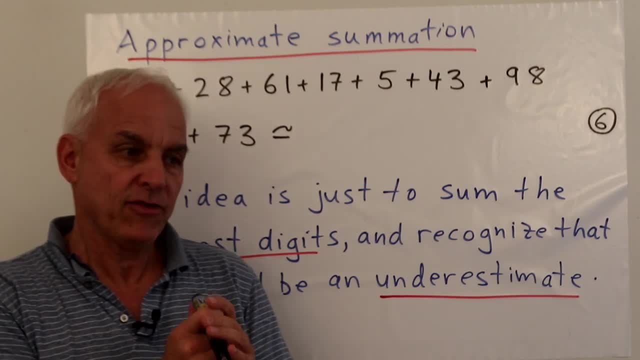 I want to say a little bit more about the number of digits. I want to say a little bit more about the number of digits. I want to say a little bit more about this approximation issue. This is something that happens quite a lot in practice, because sometimes we're only interested. 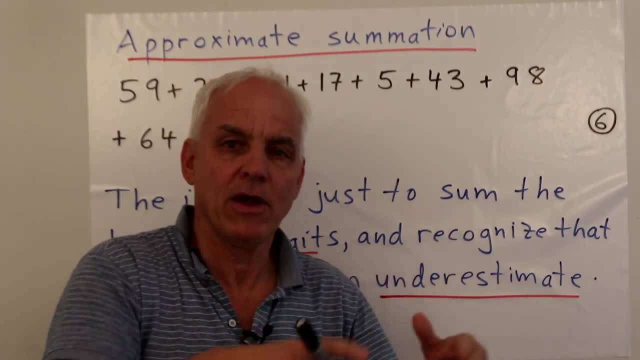 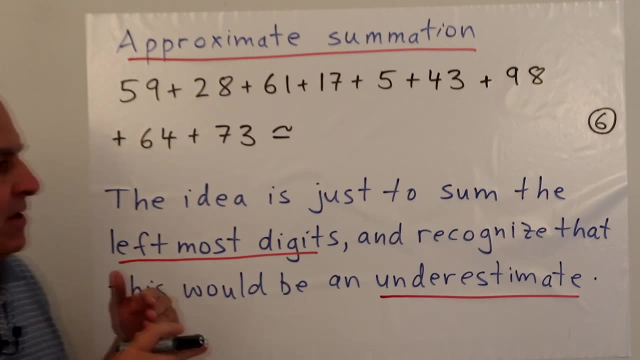 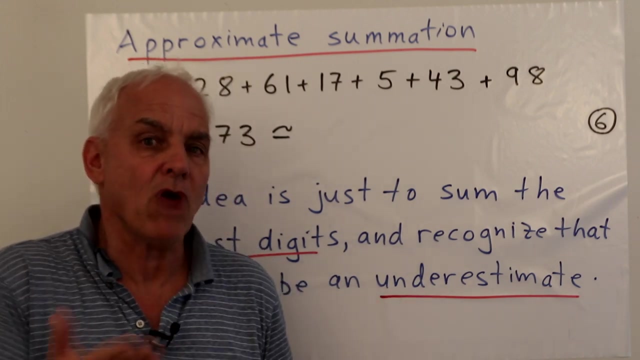 in how big or how much of something there is approximately. Maybe we don't need full accuracy, And so it's nice to have a kind of a variable or a flexible approach to arithmetic that allows us, in certain circumstances, to drop our accuracy level, And this top-end approach is very useful. 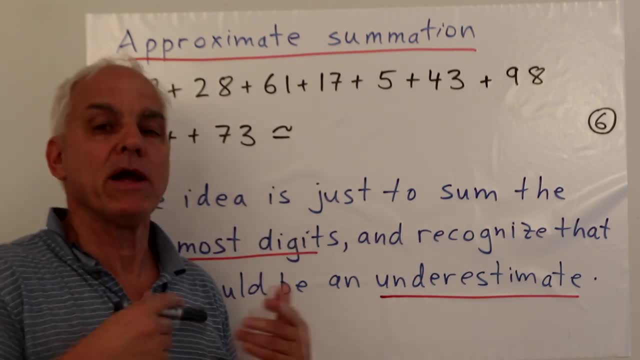 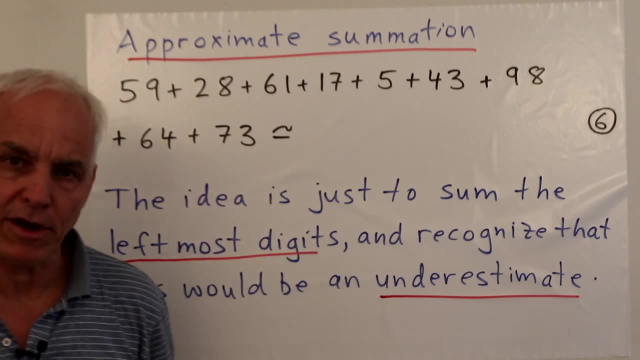 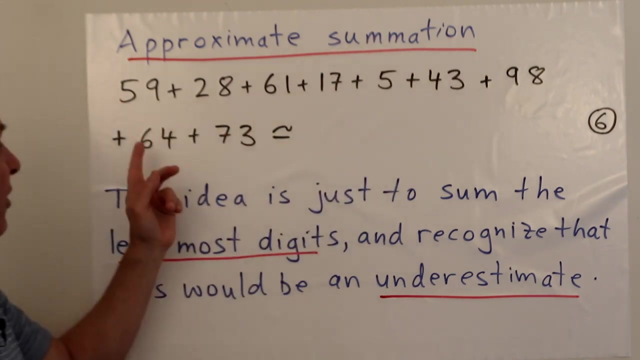 And this top-end approach is very useful And this top-end arithmetic is more in line with that. So let me illustrate that. Suppose we want to get at this rather formidable looking sum here, approximately, So we have 59 plus 28 plus 61 plus 17 plus 5 plus 43 plus 98 plus 64 plus 73.. 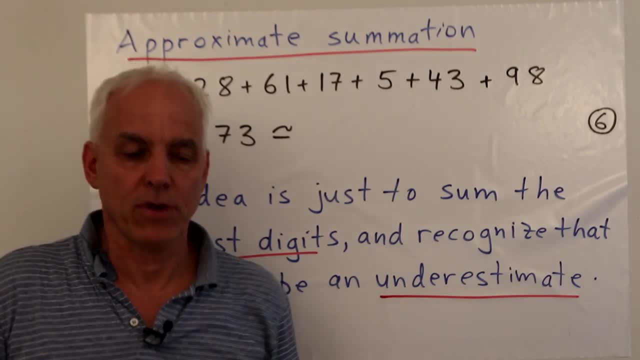 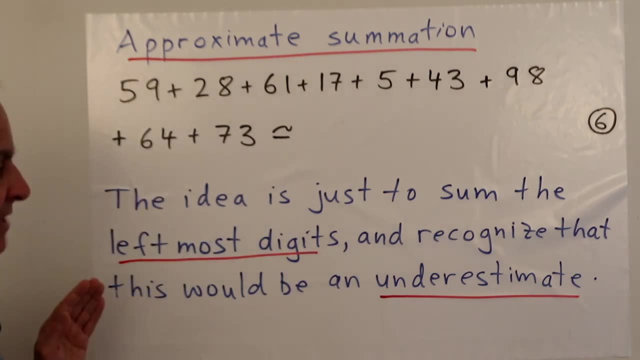 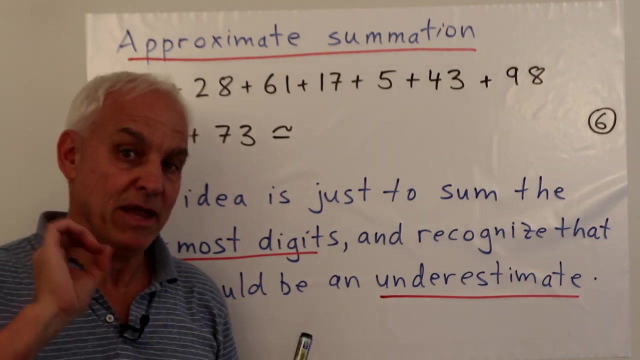 We want to know roughly what this is. okay, So it's a little bit ambiguous what that means, but let's see what we can do. So a very simple approach to this is to say, all right, we're just going to add this up, but we're just going to stick with the big end of things. 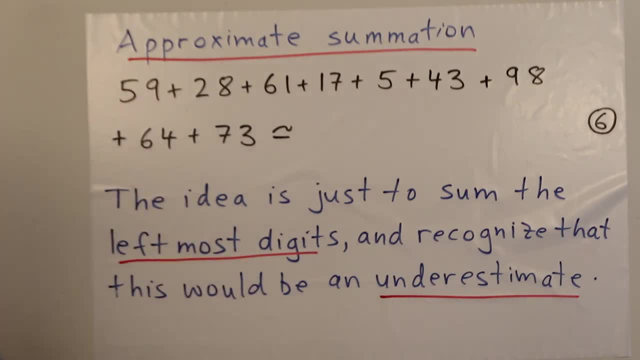 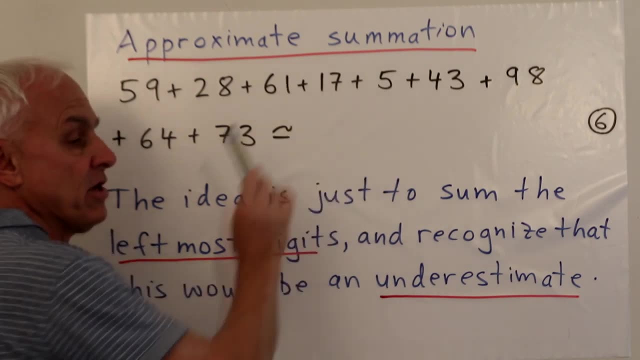 In this case the tens. So let's add up the tens: Five plus two is seven, plus six is 13, plus one is 14, plus five is. oh no, that's not plus five, There's zero there, right. 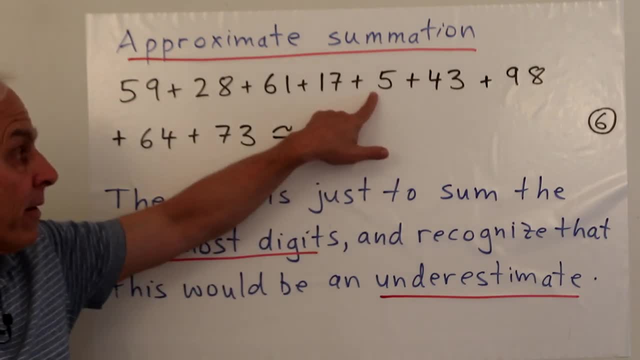 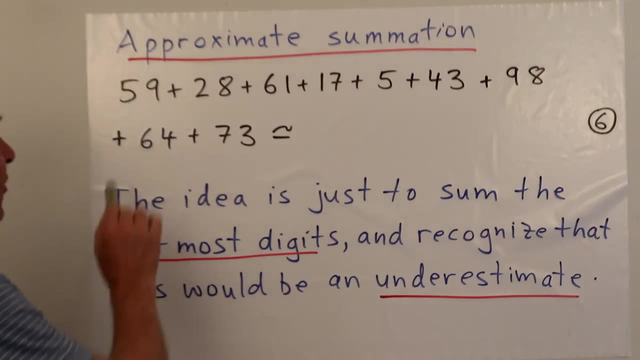 So we have 14 plus zero tens here. it's still 14.. Plus four is 18,, plus nine is 27.. Plus six is 33,, plus seven is 40. And then there will be something else when we added up all the ones. 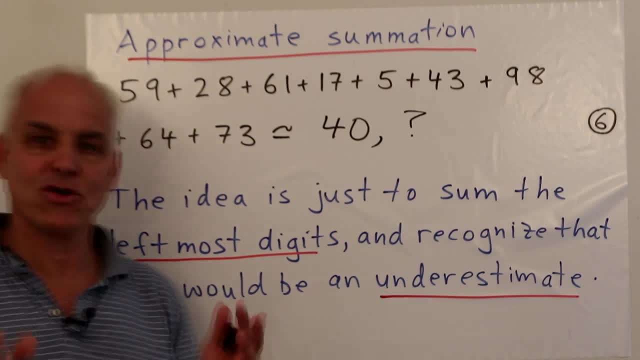 But let's not do that and let's just leave it as a question mark for now. all right, So what is this calculation doing? We haven't done the entire sum, We've only done the tens, but we know therefore that the answer is likely be something that's. 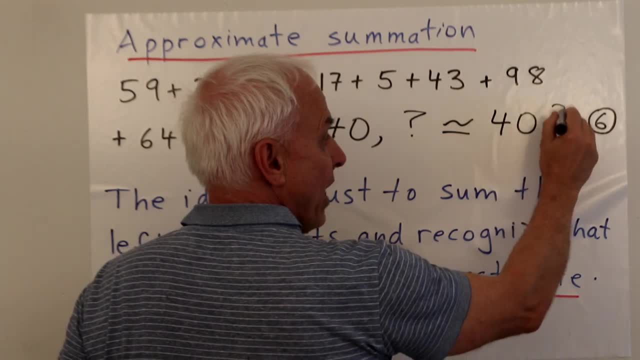 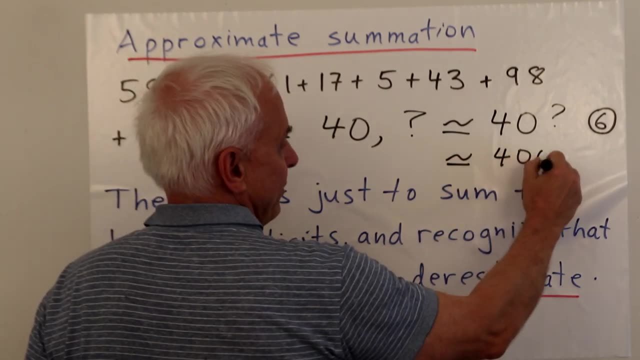 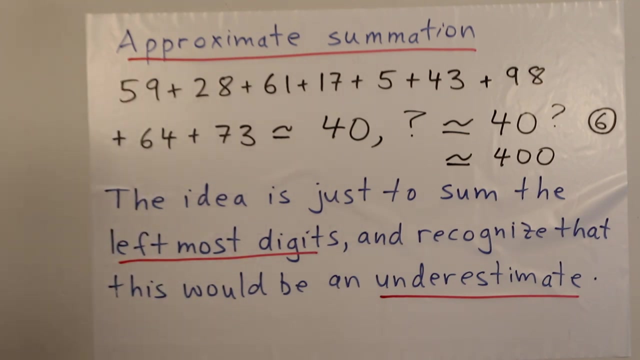 close to- Okay, 40 with another digit, So we could say it's perhaps close to 400 if we replace this final digit with the simplest possible thing, which is zero. So that's what we're doing: We're just summing the leftmost digits, but we're recognizing that what we're going to 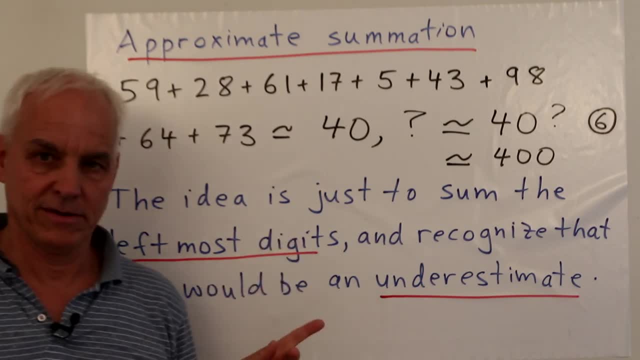 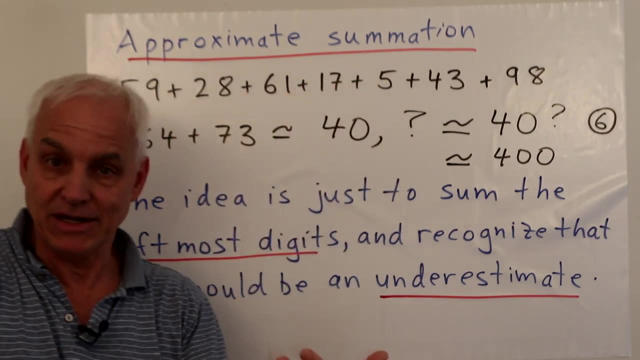 get here is going to be an underestimate. The actual, real answer is going to be bigger than that, right, Because we've dropped a lot of ones. There's going to be something in addition, But nevertheless, if we're only interested in approximately what this thing is, well, 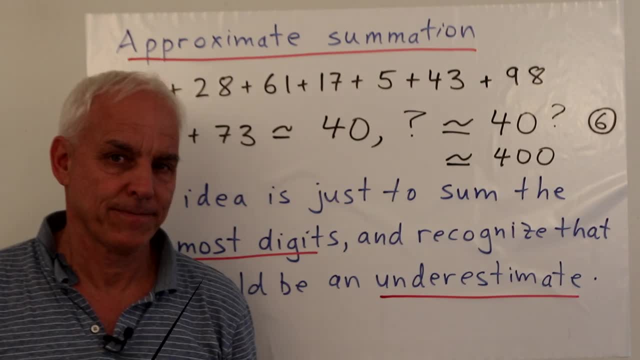 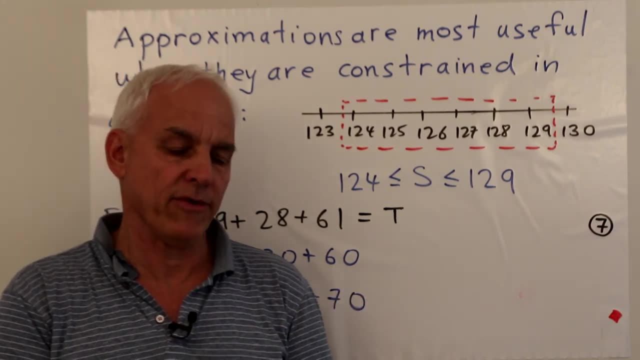 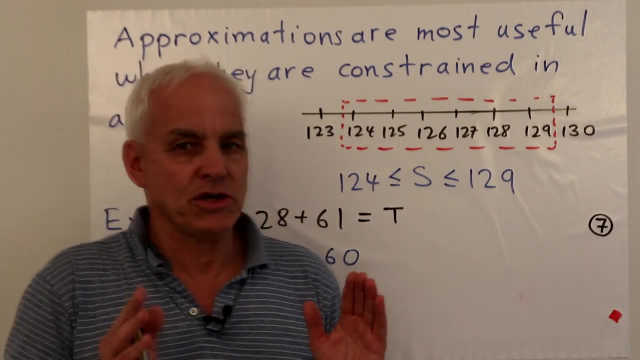 that's some kind of answer. So this is one of the first times that I've talked about approximations and just a very quick introduction to this rather important subject. But I want to emphasize even at this early stage that there's an approach to approximations. 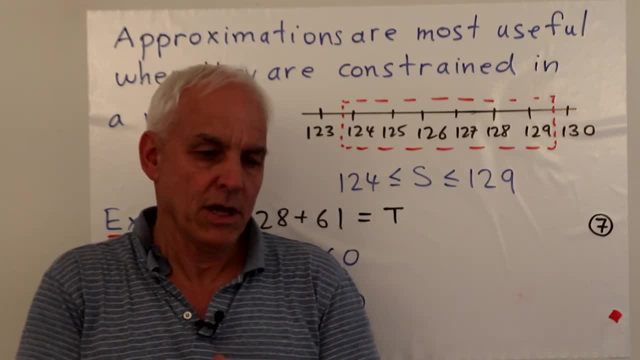 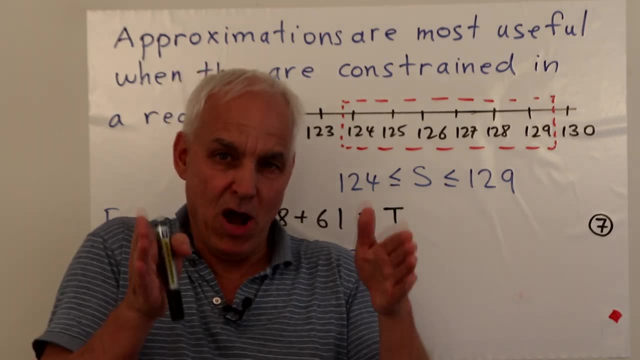 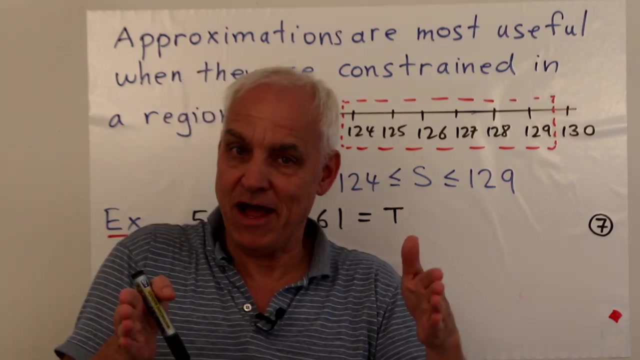 a general philosophy, which is quite good, Which is to think that, if we want to approximate something, what we should aim for is to put it in a box, In other words, to know some bounds, To know that it's between this value and this value. 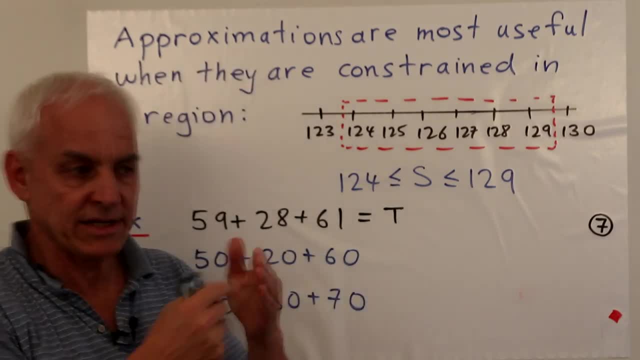 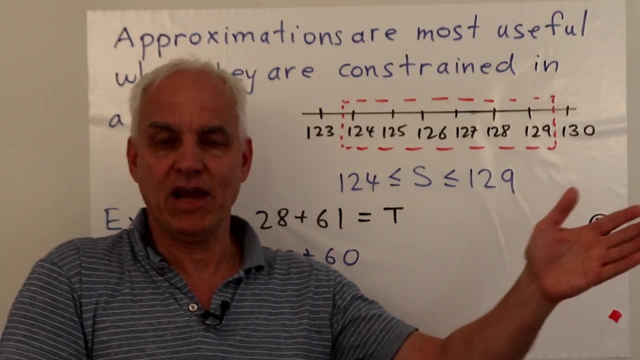 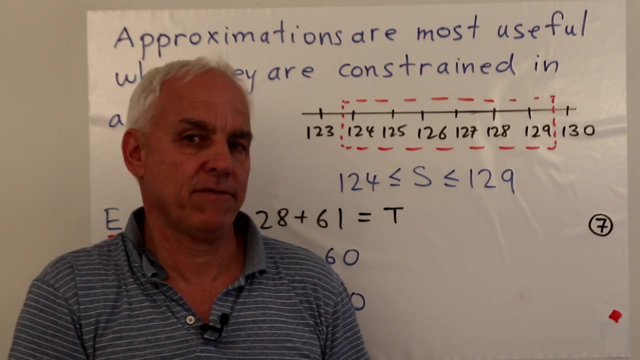 What I've just done on the previous slide tells us that we're getting some answer, but it's bigger than 400, okay, But that's a kind of an open-ended kind of statement. Okay, It gives us a rough idea, But how much bigger or what kind of bound could we possibly have? 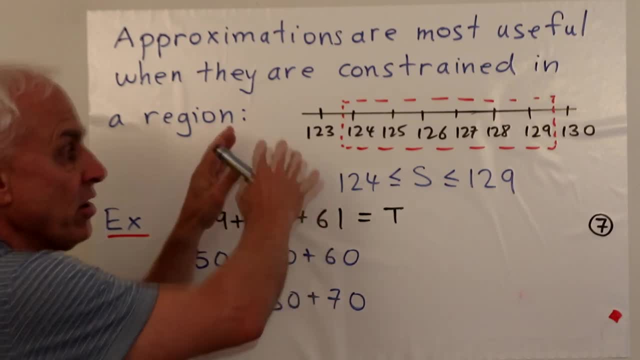 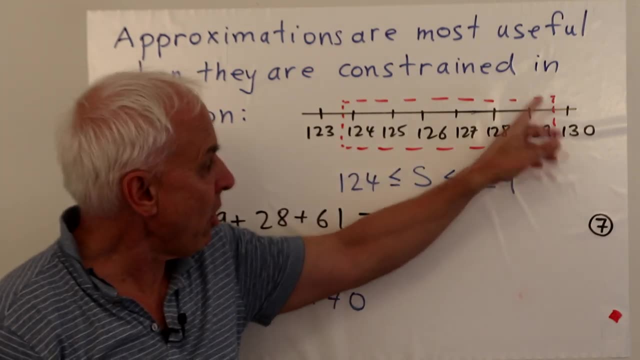 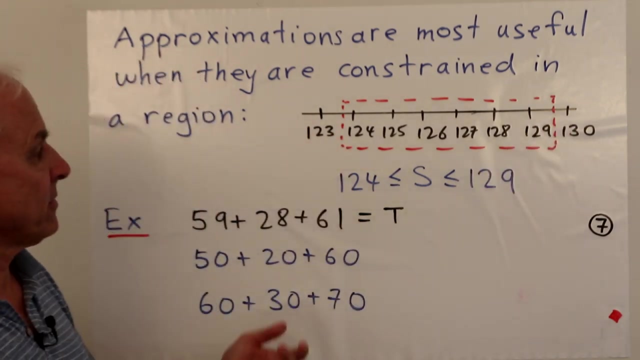 So have a look at this. This is a kind of a representation of part of a number, line 123,, 124,, 125, up to 130.. And suppose that we know that the result of some calculation or measurement is somewhere in this range. 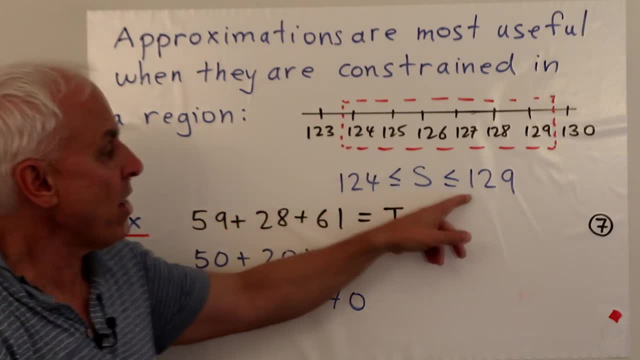 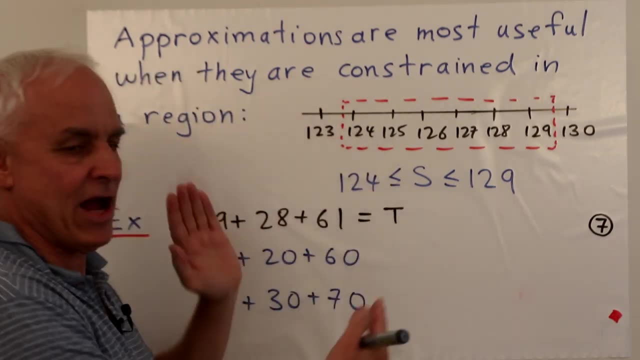 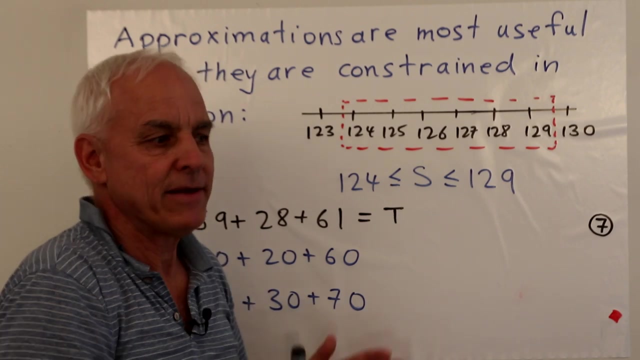 Somewhere between 124 and 129.. That's a nice kind of approximation because it bounds the uncertainty. We're saying, okay, there's a number, there's an answer. It's somewhere in this range. That limits the possibilities. 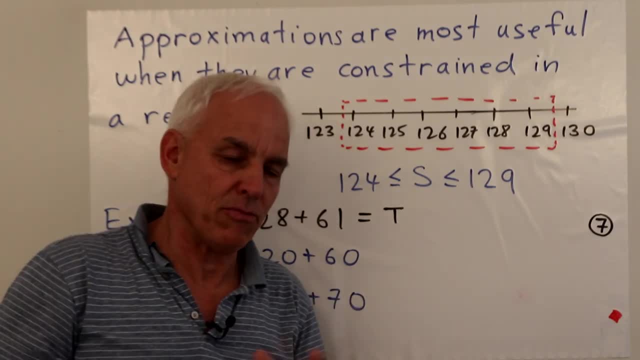 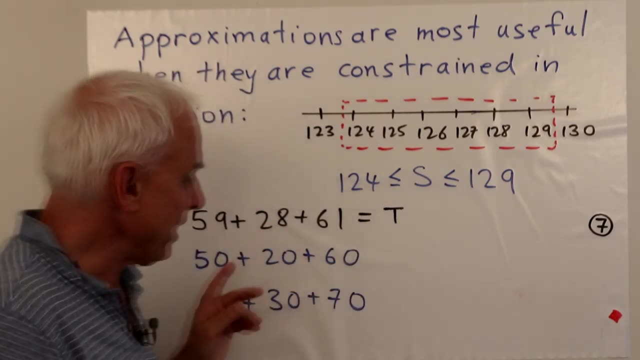 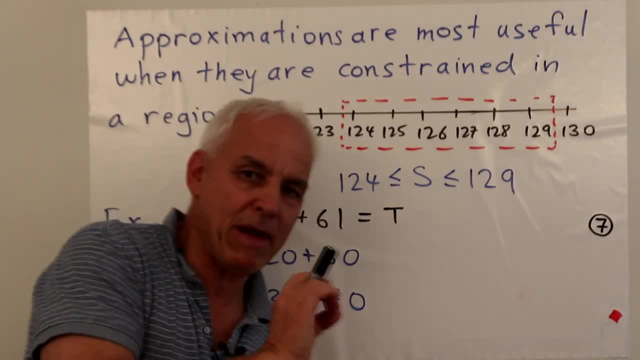 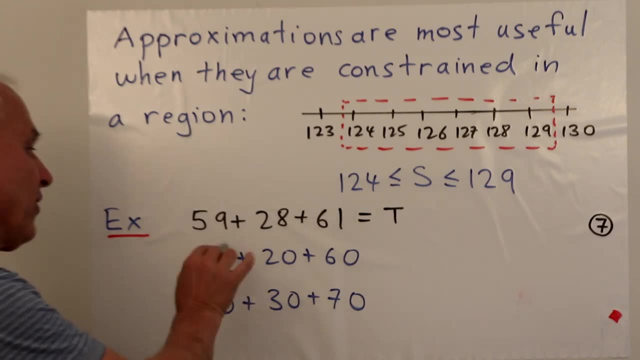 So let me illustrate that by this top-end problem. Let's have a little approach and see if we can do a little bit better than we did in the previous example, But I'm going to stick with something a little bit simpler. Here's just a sum involving three things. 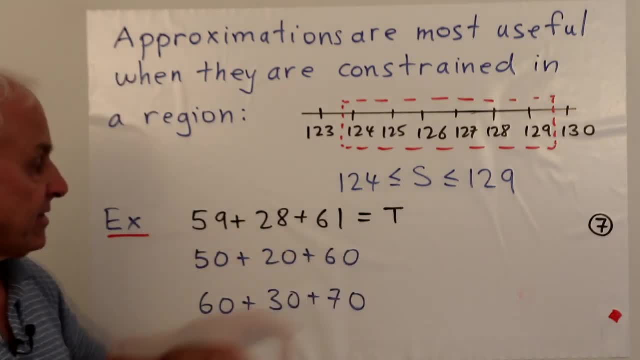 59 plus 28 plus 61. Let's say that's t. Suppose we want to do a minimal amount of work to try to guess what this thing is. Now, in this case it's only three of them, so actually we could do it simple enough. 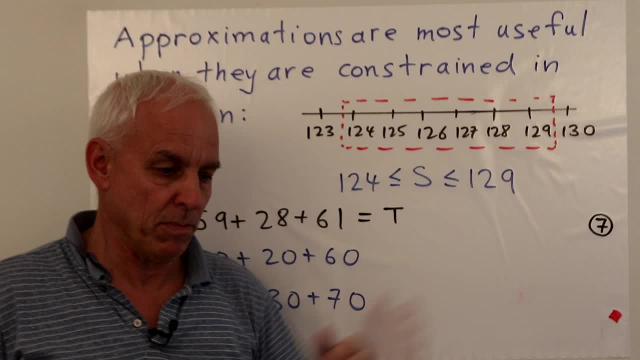 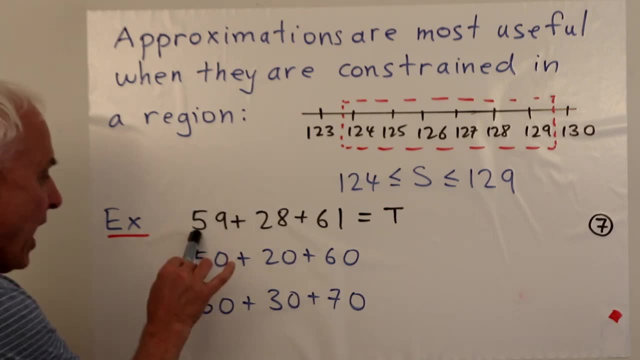 but suppose there were lots of them Doing the whole thing would be fingers Point x, y and y- quite a lot of work when we take a big end point of view. we're only looking at the tens, the five, the two and the six and adding them up. so five plus two is seven, plus six is thirteen. 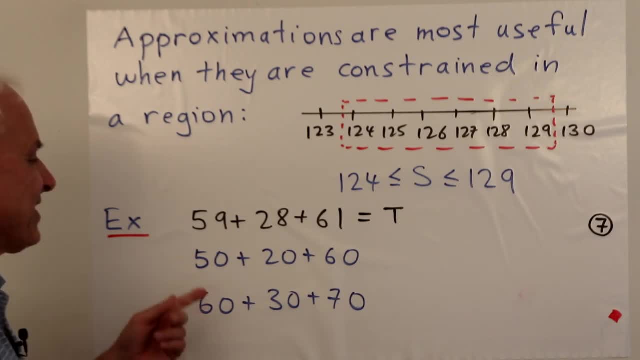 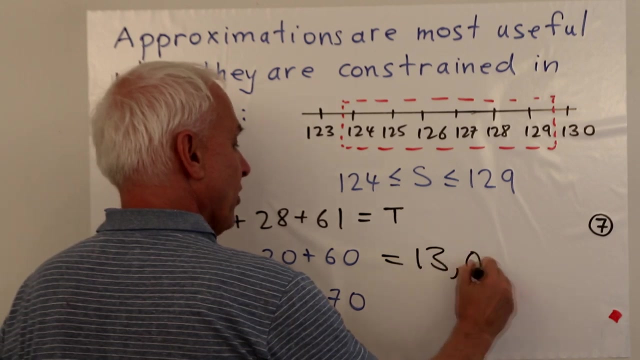 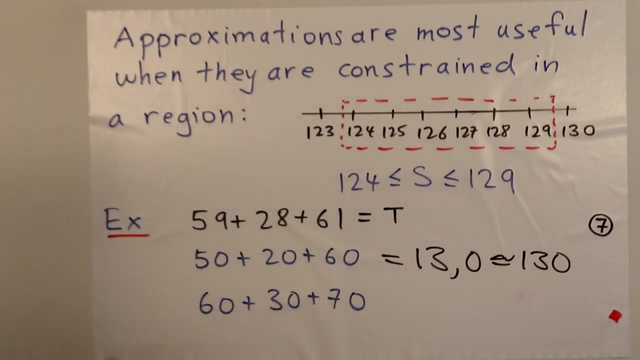 what that really amounts to is summing up 50 plus 20 plus 60. right here there's. we've sort of dropped all of the ones or replace them with zeros, so this thing actually is: five plus two. seven plus six is thirteen, so it's 13, and then zero, which is 130 or equivalent to now. that's going to be a lower bound. 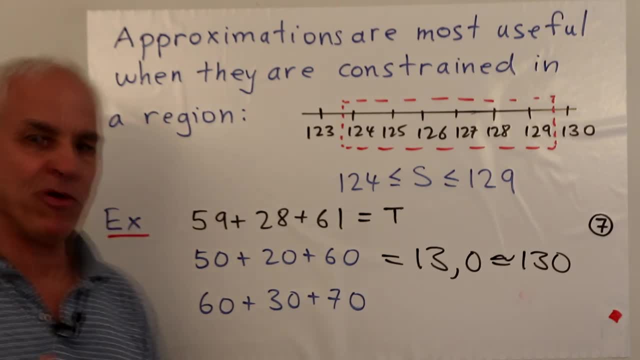 to this and i want to show you how to get an upper bound. okay, so the 59 is going to be less than or equal to 60.. just jacking up this tens value to the next value, 60.. the 28 is going to be less than or equal to 30. 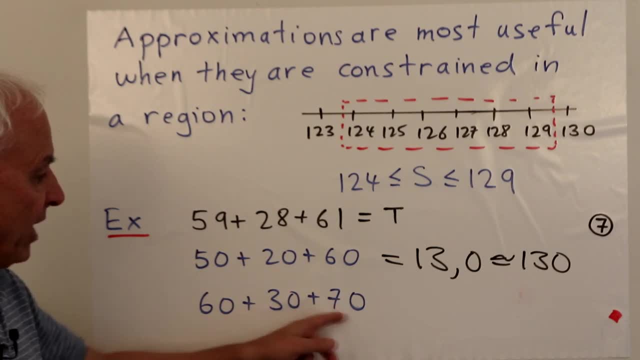 jacking up the two to a three, and if we jack up the six to a seven, we get 70.. so this is another kind of simple sum, really only involving adding up tens, that we can do easily. that will give us an upper bound, and that would be: six plus three is nine, plus seven is sixteen. so that would be. 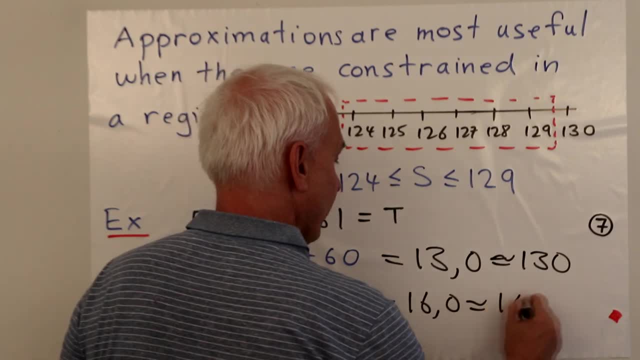 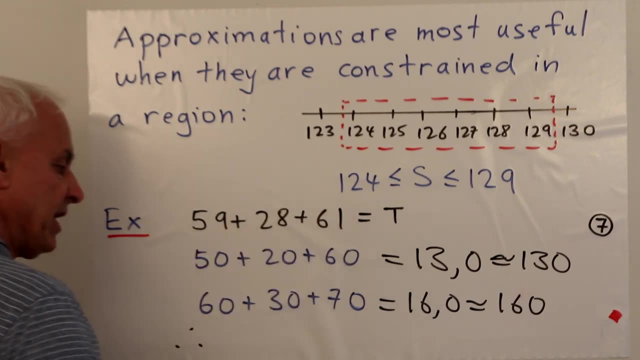 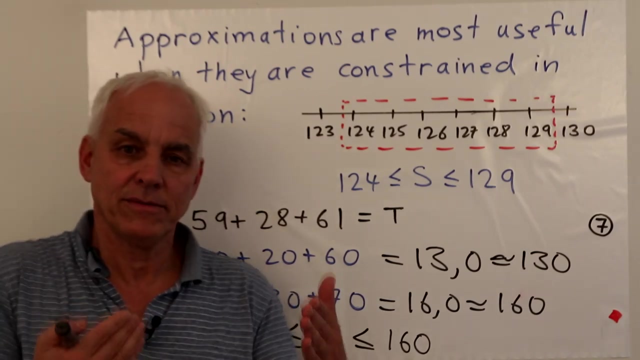 sixteen comma zero, which is 160.. so what we can deduce, therefore, is that this number t that we're interested in is actually sandwiched between, so we can use the less than or equal to sign sandwich between 130 and 160.. that's quite a range, but still it gives us an interval.